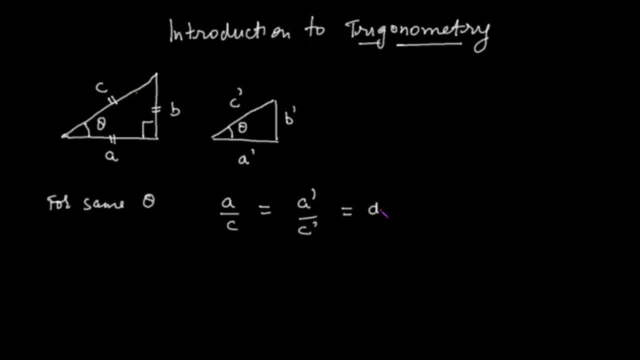 same And this ratio will depend upon theta right And that will be called cos theta. So we call this quantity as cos theta right. So for now you can just memorize this, that this is called cos theta, And as we progress in the video I'll explain you what does it really means? 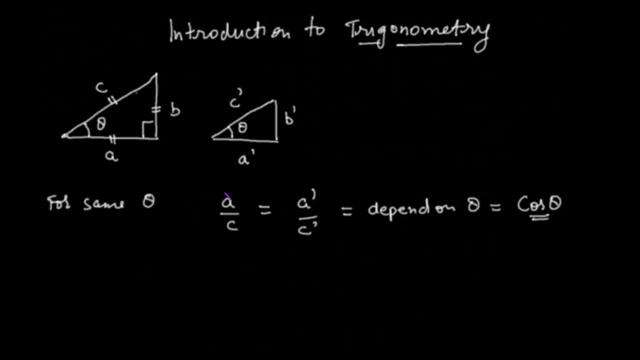 when you're trying to understand it right, But the right now. the idea is that the ratios are constant And this ratio is called cos theta. This is called theta because the it is dependent on theta and its value will change as the theta will change, right? Similarly, we have B divided. 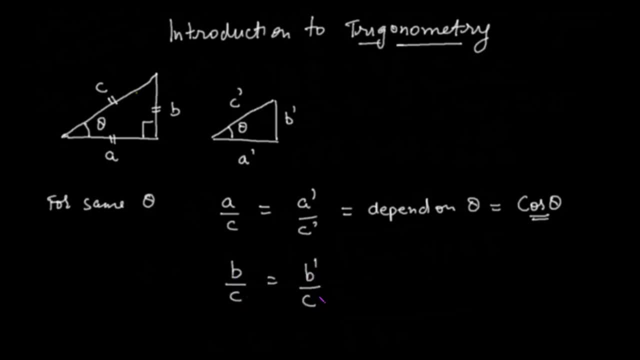 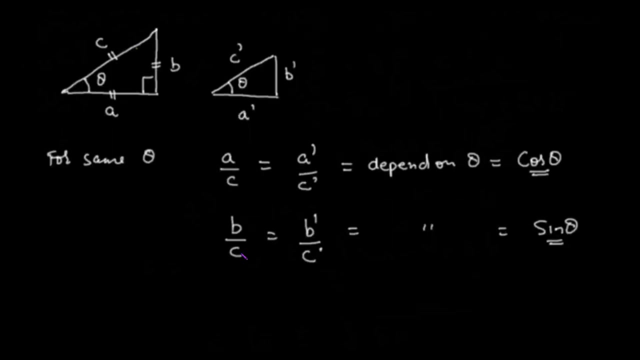 by C, And that is equal to B dash divided by C dash, And that will also be dependent on theta, And that's equal to sine of theta. And last one is B divided by A, that's equal to B dash divided by A dash, And that is equal to, again dependent on theta, And that's equal to tan. 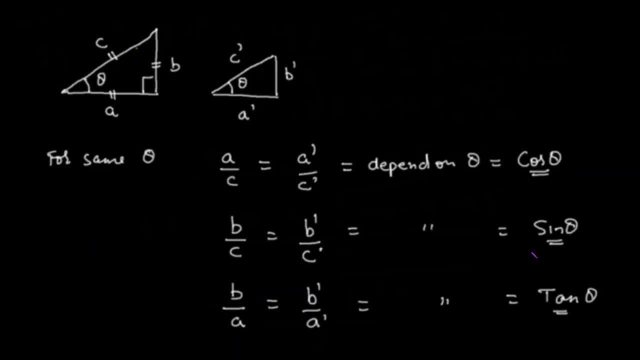 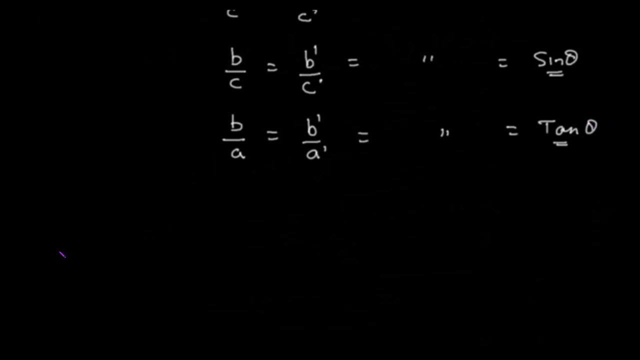 of theta Right. So these are the three quantities we need to remember, And idea is that, again, as you change the theta, the values will change. Now let me again look into it. So, as we talked about before, we have: this is a right angle triangle. Now, this is a right angle triangle. 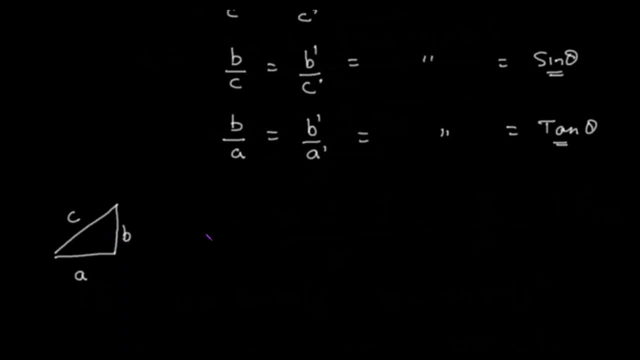 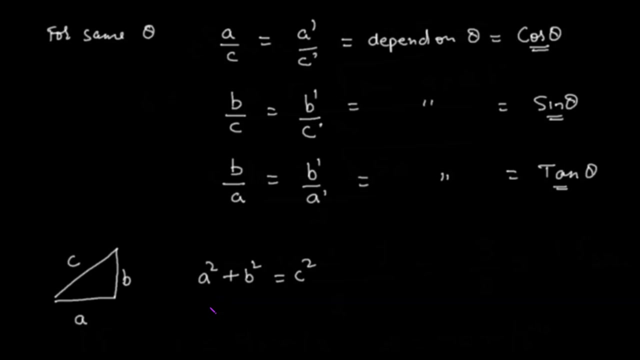 I'll draw it again now: A, B and C. So we have A square plus B square is equal to C square. So we know that right, we apply that we will have. we divide all of them with c square, so we divided by c square. 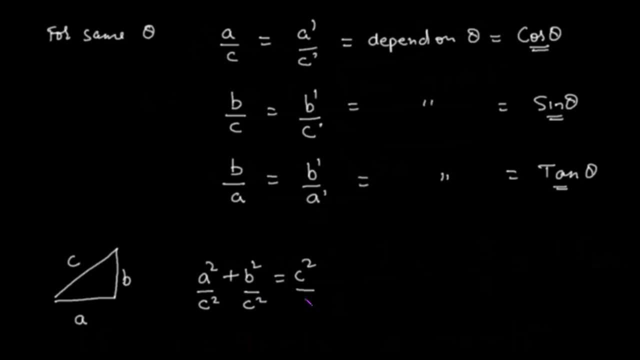 so if i divided by c square, c square and c square, that will give me one, and a square divided by c square is equal to cos square theta plus sine square theta. so we have this relationship: that cos square theta plus sine square theta is equal to one. 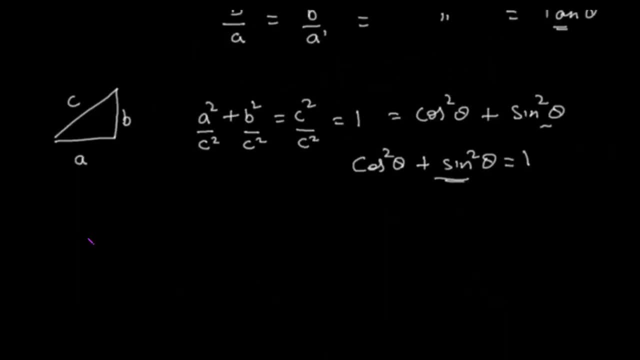 so that is a important relationship when it comes to trigonometry, right? the another relationship which is important is now: look at this triangle now. this is theta and this is 90 minus theta, the other one right. so one of them is theta, the another one is 90 minus theta, right? so 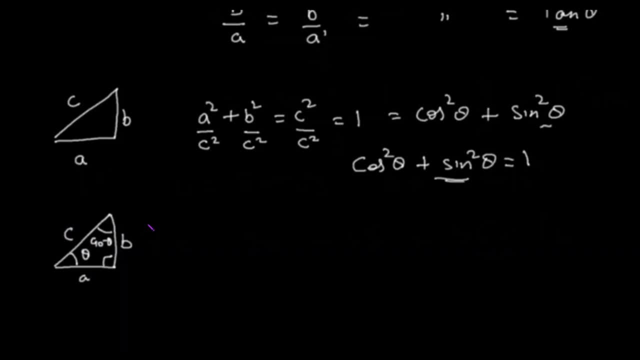 this is b, a and c. so how about i flip this? so if i flip this, then this will become like this: this is 90 minus theta and this is theta. and because we flipped it, now this is b, this is a and this is c. now think about it. in this case, we said that sine of theta is equal to. 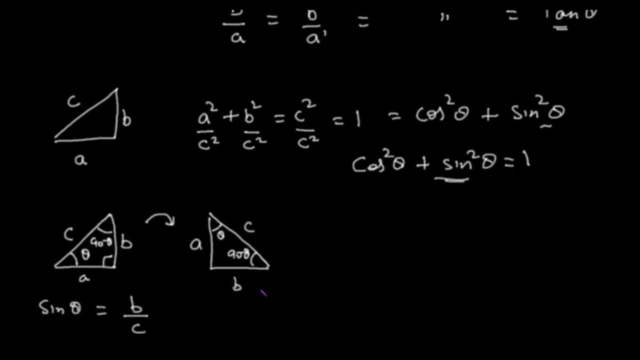 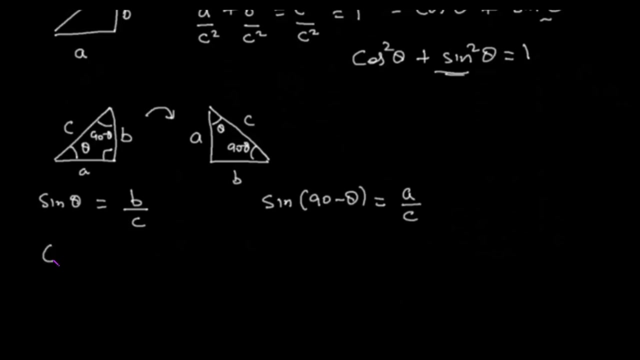 b divided by b, c. but here we have sine of 90 minus. theta is equal to a divided by c. right, right. and what is a divided by c but a divided by c? if you look at this triangle here, cos of theta is equal to a divided by c. 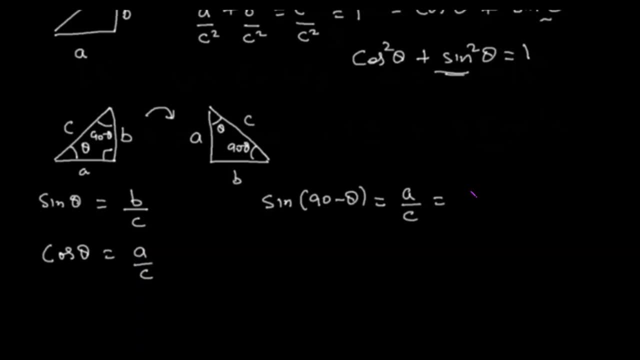 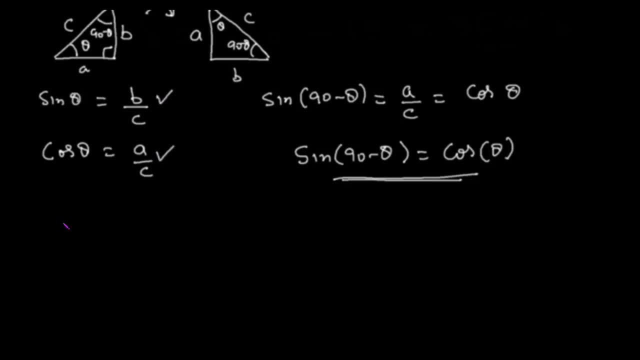 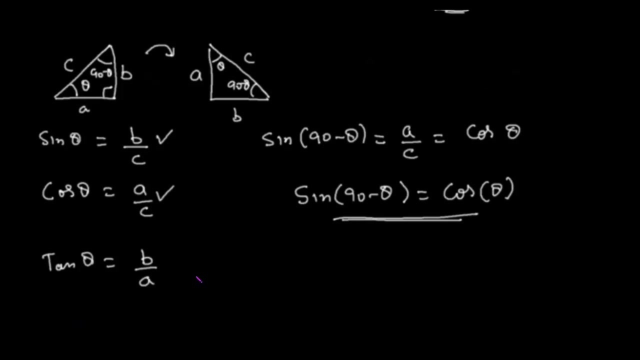 theta is b divided by c. cos theta is a divided by c. and what is tan theta? so tan theta is equal to b divided by a right, as we did before. so b divided by a. now in this case we can also write it as sine theta divided by cos theta. so this is a third relationship which we may have to remember. 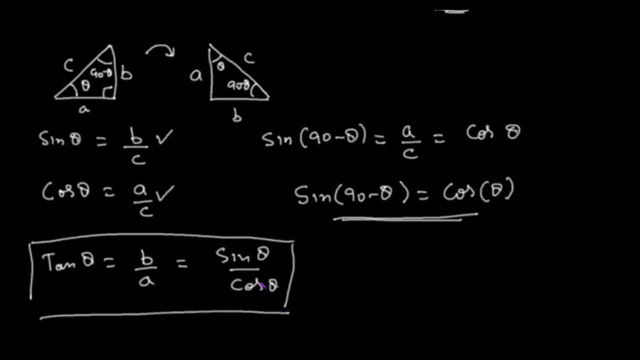 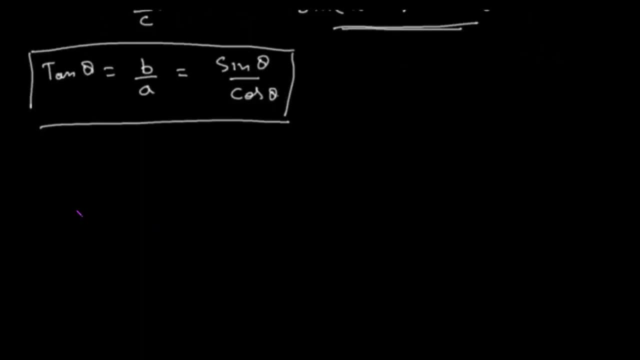 that tan of theta is equal to sine theta divided by cos theta right. so these are basic relationships. now, why do we need technometry, right? so now, let's say that we have a force. now, suppose, if you are mowing the lawn right, so you are mowing the lawn and this is a lawnmower. 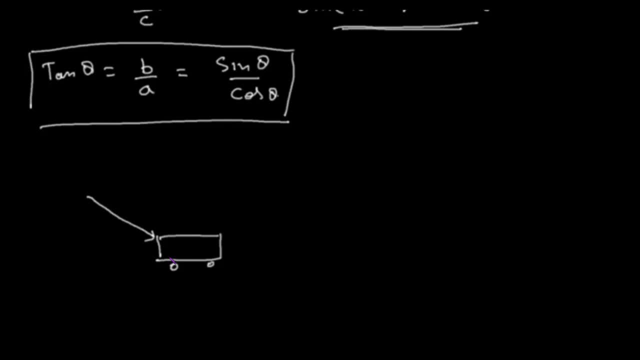 right and you are mowing the garden right. so you are putting the force on this lawnmower right now. when you are putting the force on the lawnmower, you are putting the force at an angle right. so when you are putting it at angle, this force is going into the ground right part of it. 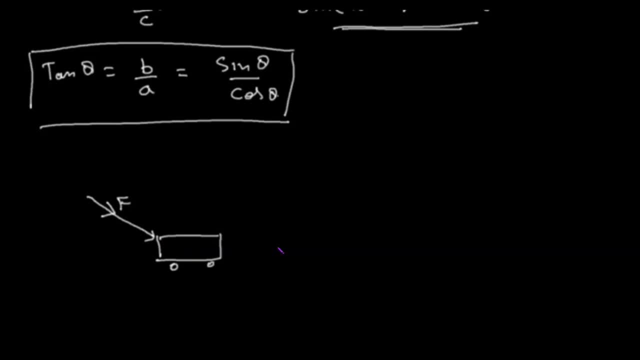 is going into the ground. part of it is forcing the lawnmower to move forward, right? so in this case, let's say that your angle here is theta, right? so what we can do is we can use the technometry to determine the force on the lawnmower. right so we can use the technometry. 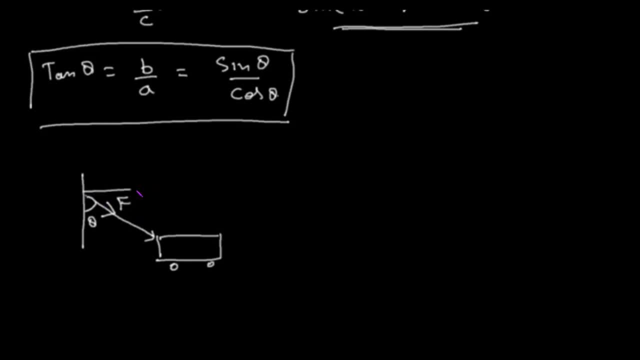 divide this force into two direction. one direction is this and another direction is downwards- right, so let me draw this again. so this is a force, right? so we take this and make a triangle out of it and we call this as right. so, and and let's say, this is theta, so 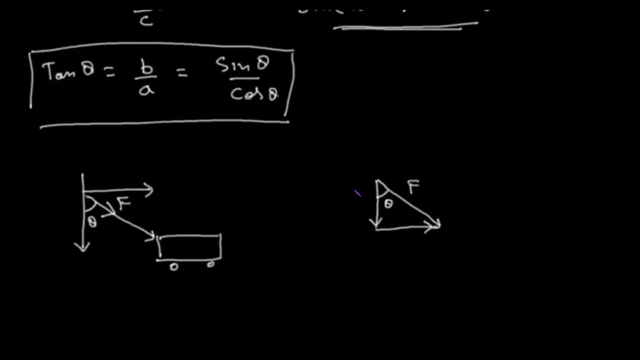 if this is theta and this is f, then this quantity, this quantity will be equal to right. so let's call, let me call this as f? y, because this is in the y direction. right, so f of y will be equal to f cos theta. right, because in this case, in this triangle, cos of theta is equal to f of y divided. 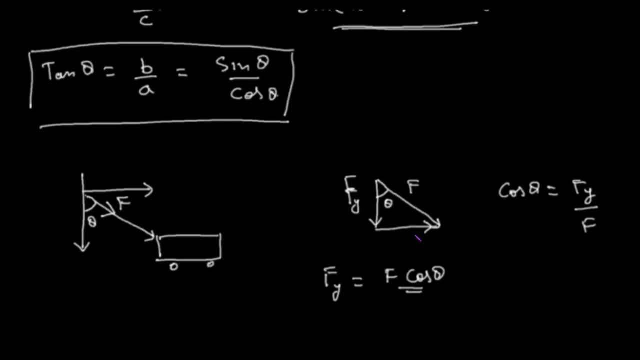 by f right and similarly this one, which is f of x, that will be equal to f sine theta, because sine of theta is equal to f of x divided by f. now we can draw this again and we can draw it like this, because this this line, we can move here now, we can keep this line here, but we 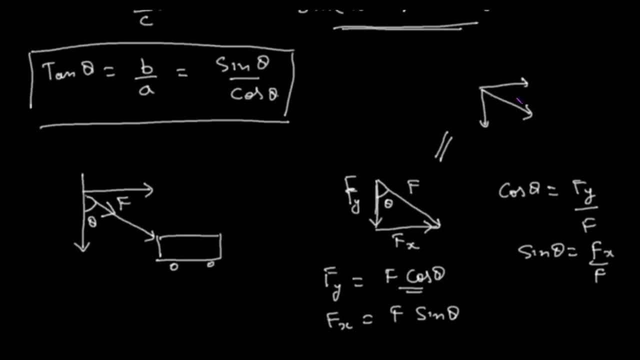 let's move the fx here right now. what you did was you divided the force f into two parts, f of x and f of y, right? so technometry help you divide the forces into two direction, right? this is one of the application of the technometry. so we, how do we know the cos, theta and sine theta? so we have a table. 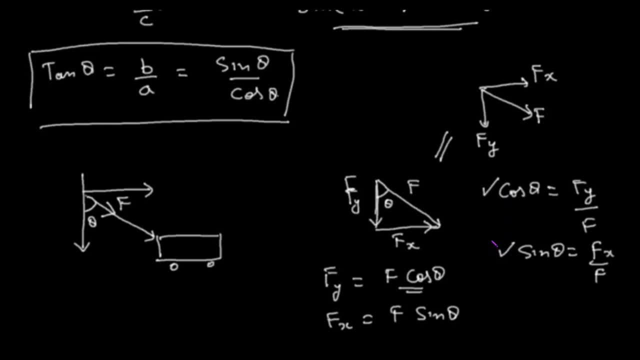 where we already measured how this ratio changes with the theta right. so we have a, so for each theta we have a value of cos theta and value of sine theta. so we can use that table and we can find out what should be the relationship between the x component to the actual force. 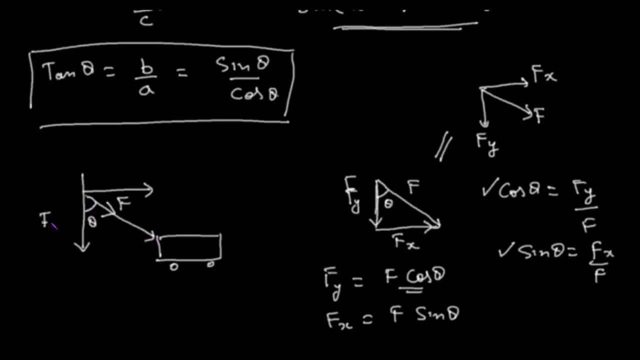 which was applied on the lawn mower right. so based on that we can calculate f of y and f of x right. so only the f of x will move this lawn mower forward, but f of y will only be pushing it down into the ground. right now, this is one application. another application. 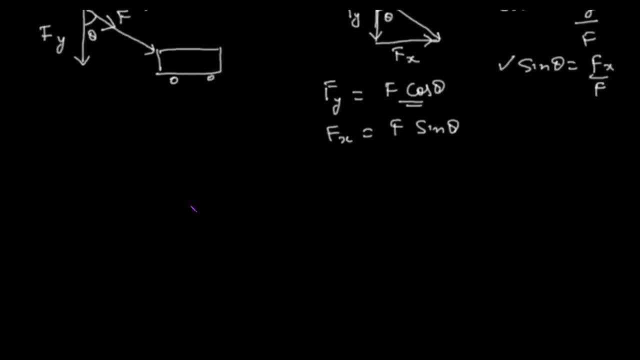 is suppose if you are standing here, you are standing here right and you are looking at a building. so this is the building right, you are looking at the building. so when you are looking at the building, you can look at the top of the building. so when you are looking at the top of the building, 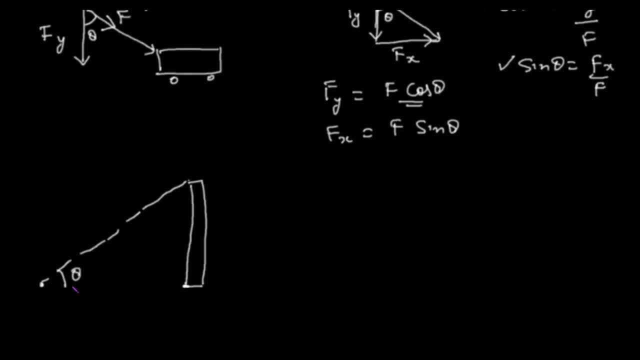 right. so you know that, what angle you are looking at. if you are not sure, what you can also do is you can point out, you can use certain kind of instrument which will tell you at what angle you are looking, or suppose if you are looking using a looking at telescope or something. 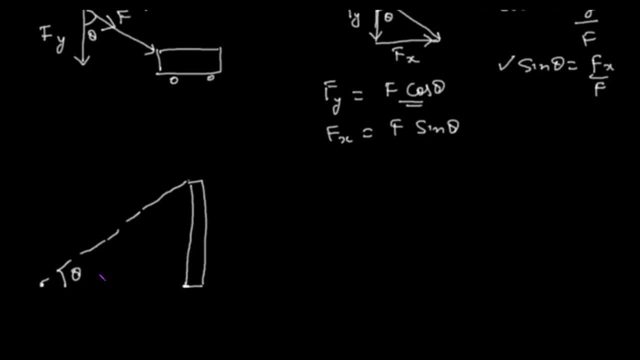 similar. so it will tell you at what angle you are looking at that building right. so you look at the top of the building, so from that you can calculate the value of theta right. so if you calculate the value of theta from there and you already know the height, 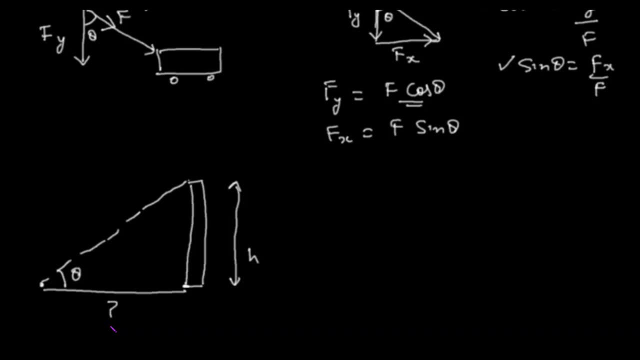 of the building right. so from there you can find out how far you are away from the building. so that's a very basic example of how you can use trigonometry, in this case right. so this is another example. so we have, we know height, we know theta and